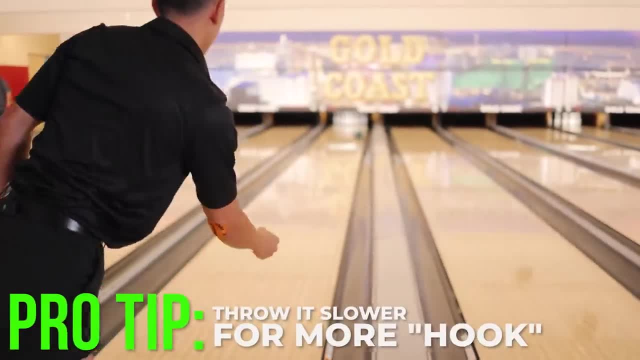 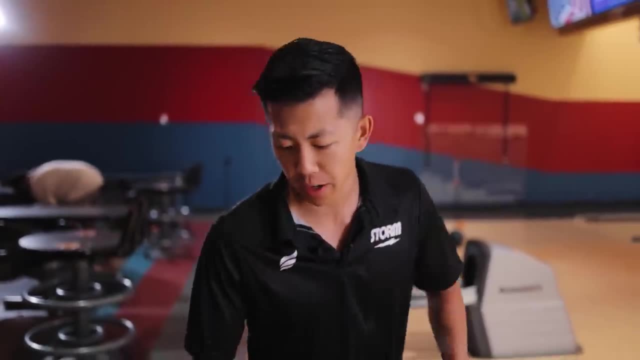 this, It's ball speed. You might be throwing it a little too hard, So if you want to see your ball cover more boards, try throwing it a little slower. Now we have method number two, fairly popular amongst mostly guys, but a lot of girls are trying to get into it. It's the two finger. 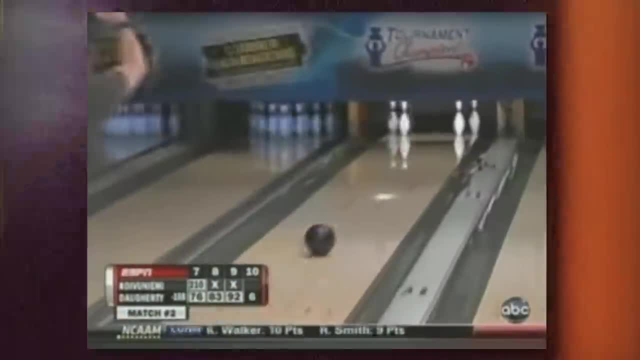 no thumb. I like to call it the Dougherty method. Those of you that don't know that he's famous for shooting 100 on TV, but still a phenomenal bowler. So what you're going to do is put two fingers in. 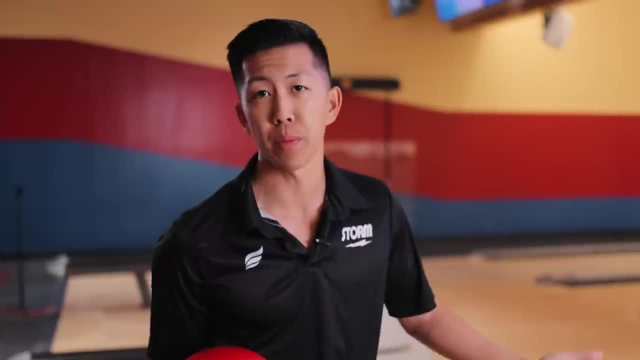 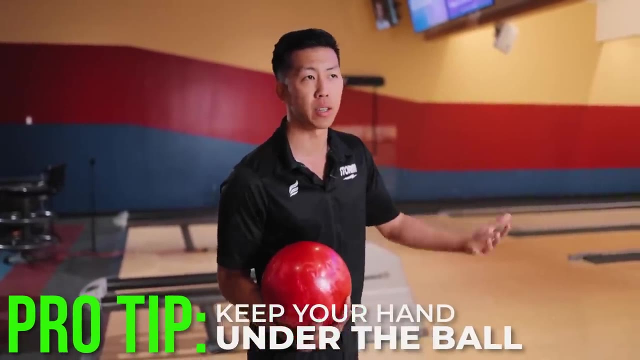 the ball, but no thumb, You're not going to use your other hand either. Actually, some people start with their hand on the ball and then it comes off. Just get your hand underneath. the bowling ball Helps you increase rev rate, So that really adds to the axis rotation and ball speed creating hook. So we're going to give it a. 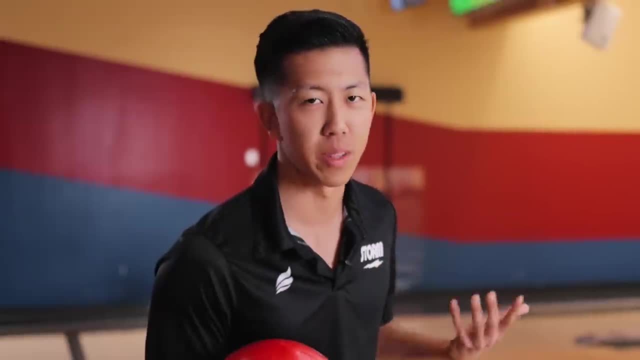 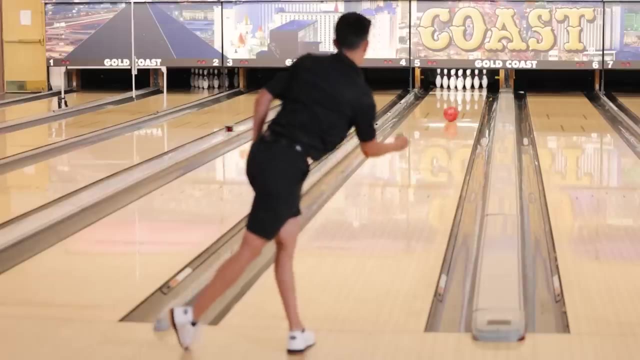 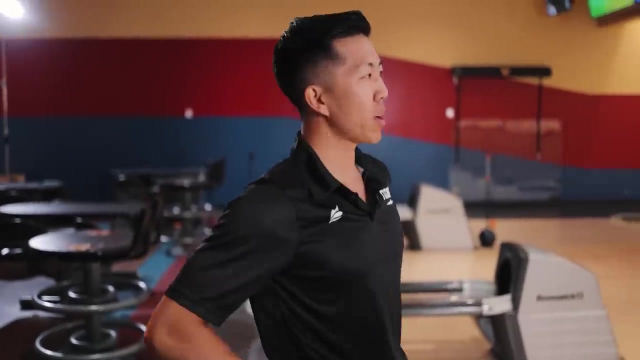 try here with a house ball. I like to use a lighter one because I'm not very practiced with this, So it makes it a little more difficult for me. Here we go And, like I said, not very well practiced with that, but, as you can see, plenty of board coverage creates a little more power. 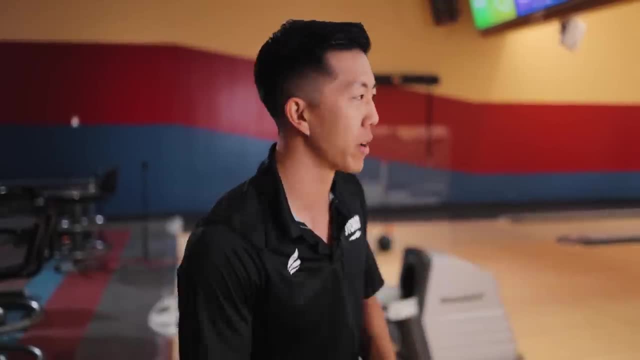 than the suitcase method. Naturally, a lot of guys you want to go for a lot of power, want to go for a lot of hook, much more hook than suitcase method. So one of the most important things, if not the most important thing. 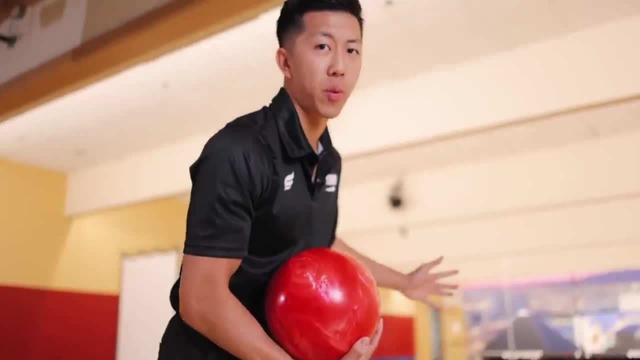 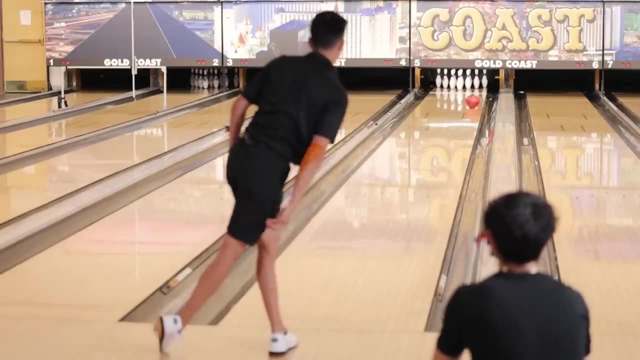 is to make sure you keep your hand underneath the bowling ball. You don't have the support of anything else. There's no anchor, there's no thumb, there's no second hand, Cup and wheel, I like to call it So. that's just two methods so far on how to hook a bowling ball, but there's. 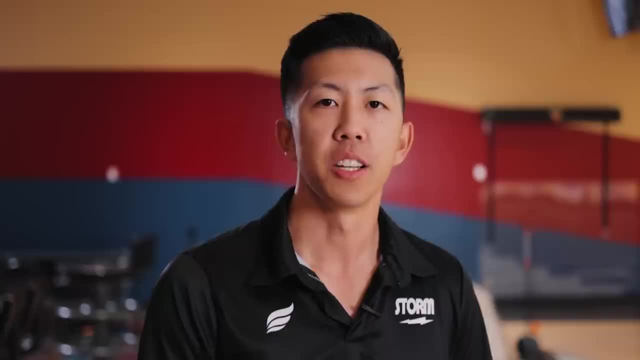 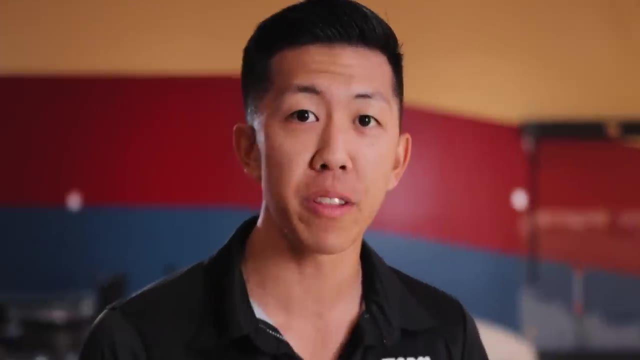 no way that we can cover everything about bowling in just one short video, And so we've launched the number one online bowling masterclass: Bowl Like a Pro. In this course, there's over 40 videos covering everything that you need to know about bowling, covering anything from fundamentals to 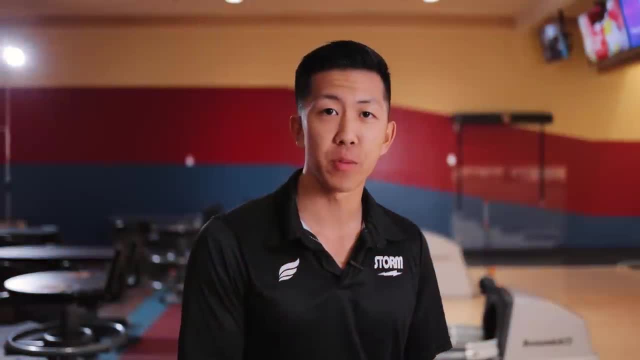 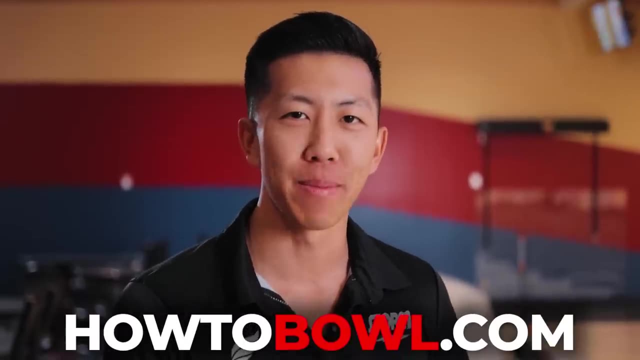 competition strategies and even tips from other pros. If you're watching this when this video goes live, the course is currently on presale, but if you're watching it sometime in the future, the course is already live. So go to howtobowlcom to sign up for the course and take your game to. 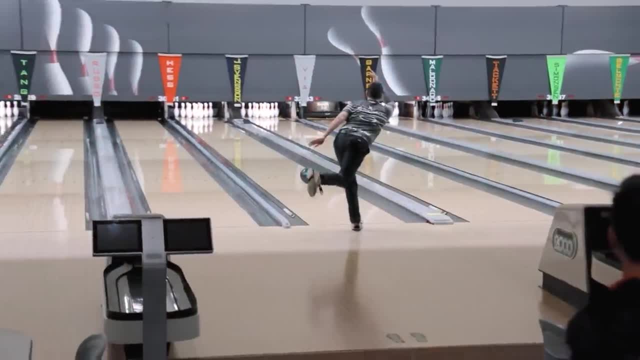 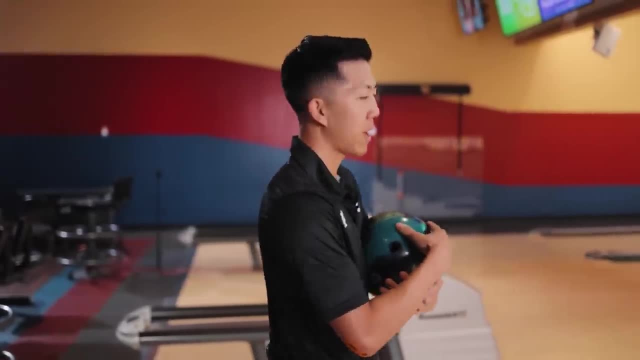 the next level. Method number three, two-handed, Widely popularized by Jason Belmonte, Oscar Palerma- you can call the OGs- kind of stepped under the pro scene, made it really, really popular, had massive success. And now we've got the younger generation, even guys who are 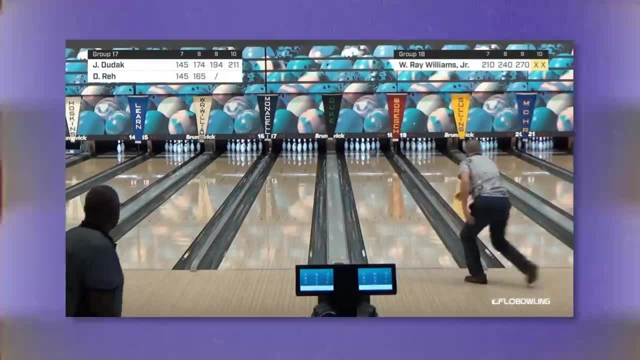 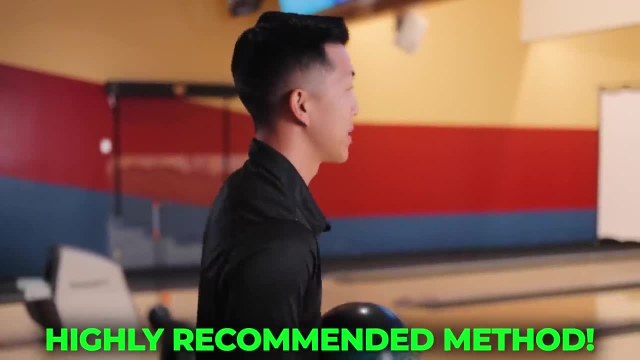 around my age, even Walter Ray trying it out. So he shot 300 ball in two-handed and he's an OG, you know. But anyways, the most popular style. I definitely recommend it if you're taking this game serious. It just takes a really big variable out of the game, which is the thumb. 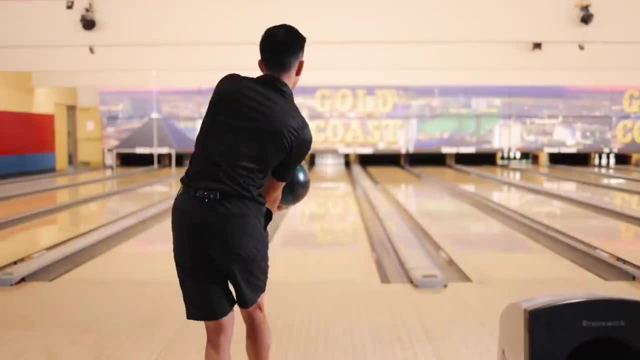 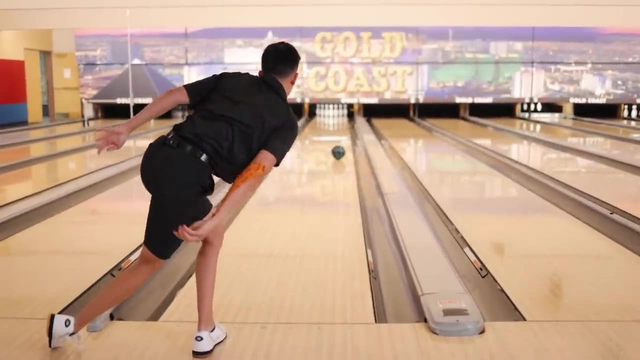 God, I wanted that to strike so bad. What you're going to do? you're going to use just two fingers, just like the two-finger no-thumb style, but you're adding the other hand of the ball, Now left hand, to act as anchors. you know, That's what keeps the ball nice and secure. So key things you. 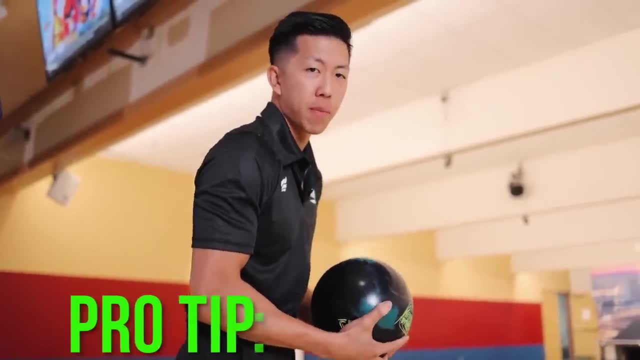 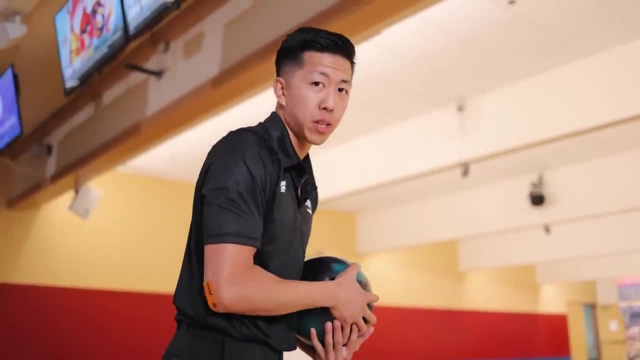 want to think about when you're bowling two-handed- more or less the same as two fingers and no thumb- just make sure you keep your hand nice, and under the ball You're going to create reverie seamlessly. And again, it's all about ball speed and axis rotation. for how much you want the ball, 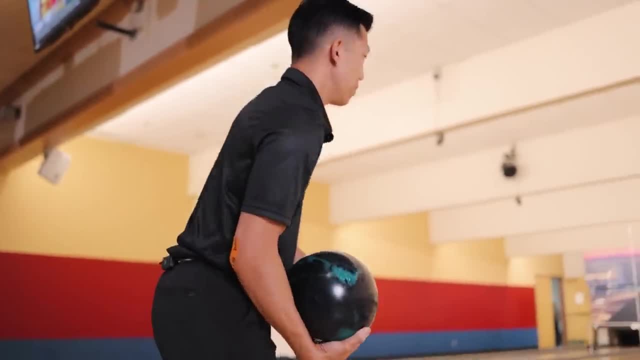 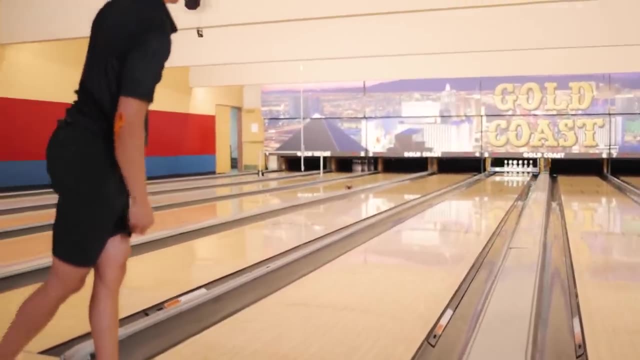 to hook. So here we are. Only difference is we have our left hand on the ball. Now we're going to throw one. Wow, Maximum hook Method number three: two-handed. That's what keeps the ball nice and secure. So here we are. Only difference is we have our left hand on the ball. Now we're going to throw one. 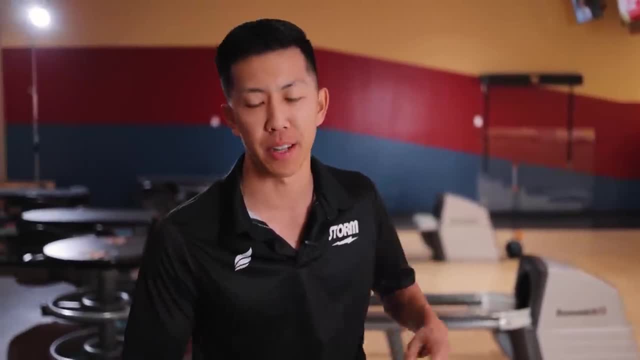 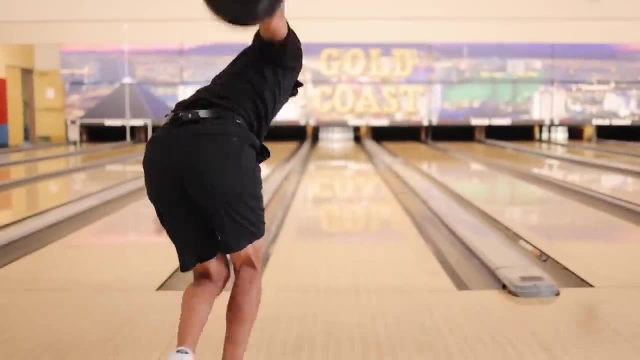 Number four: this is going to be the hardest one to master per se. It's going to be the traditional thumb in free swing style. Now, this is what I do. This is my go-to. This is what I've been nurturing for the last 20 plus years. There's a lot of different ways to go about this one. 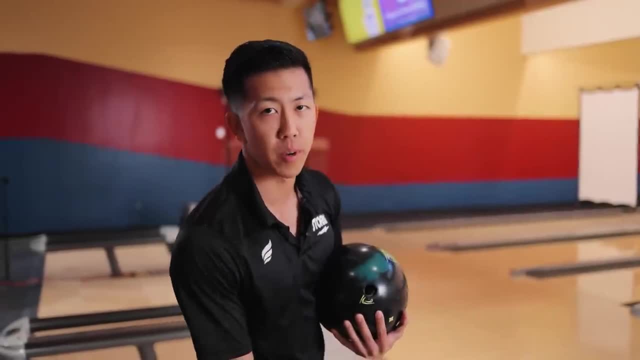 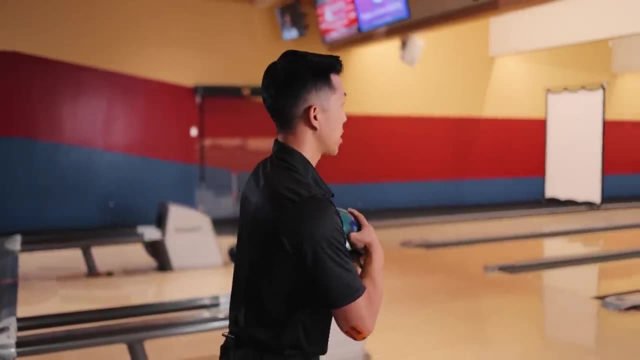 but it all kind of points towards the same thing. You want to try to get your hand as underneath the bowling ball as possible, But again, if you want to create shape, hook, it's all about speed and axis rotation. So we're going to show you how much we can hook a bowling ball with a thumb in. 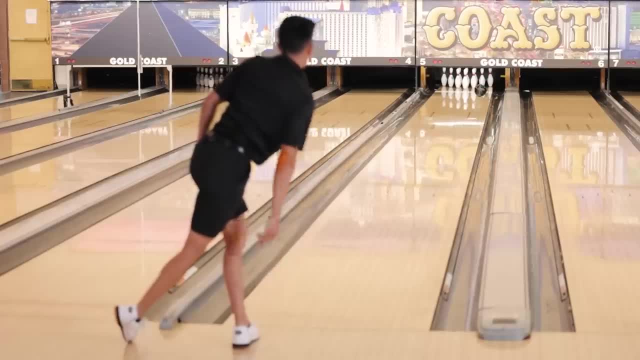 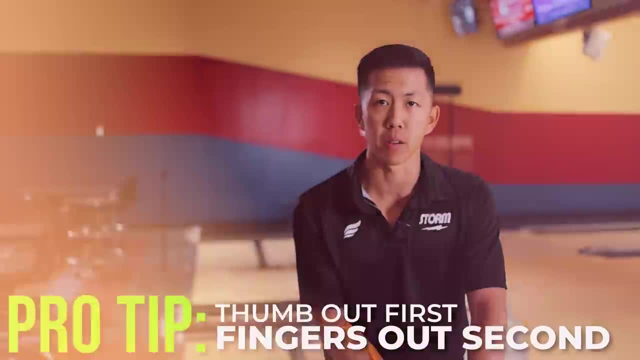 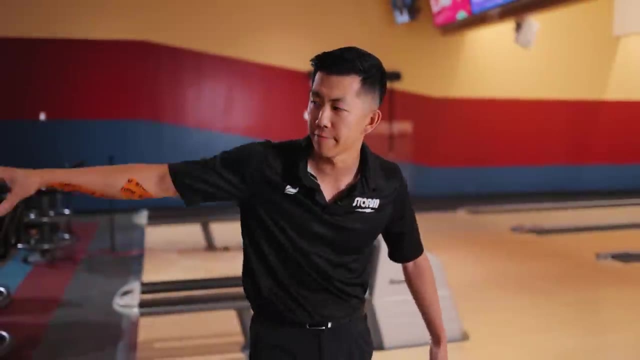 Now again, the biggest thing that I have to stress: when you're using your thumb, you want the thumb to come out first and then the fingers. Your fingers should be the last two digits leaving the bowling ball. whether it's two fingers, no thumb, two-handed or free swing. thumb in You. 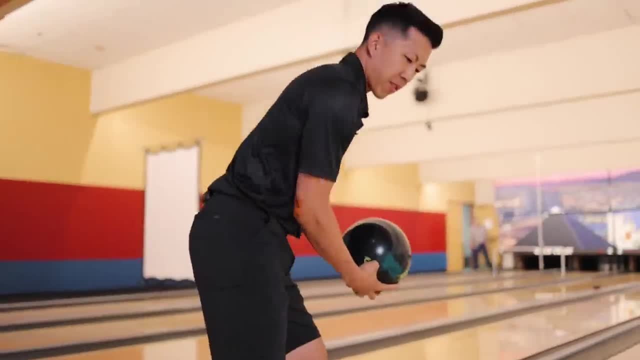 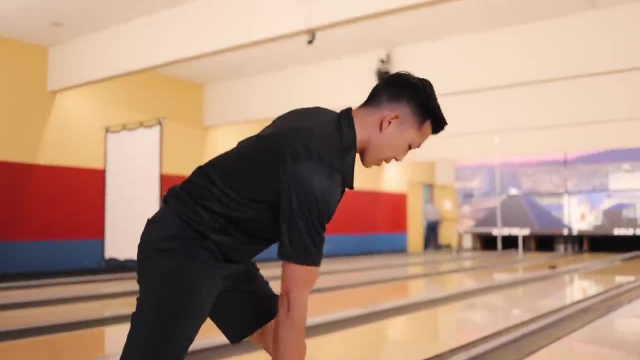 want that thumb to come out. It's going to be fingers at the end, All right, So ideally we have our hand nice and up the back It's all the same. really, The release is more or less the same, just different methods to get there. You want to keep your hand nice and under it Get your fingers.